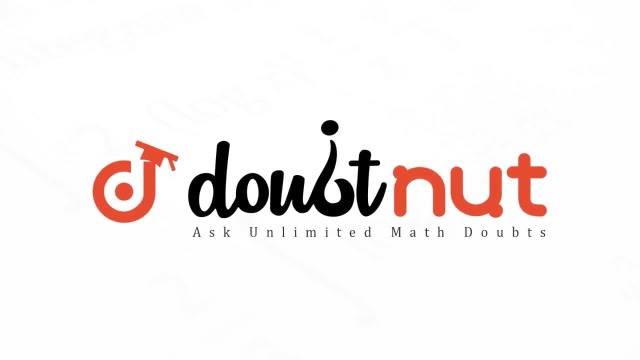 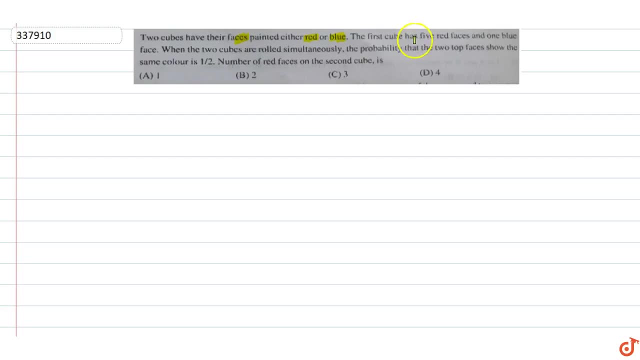 In this question. the two cubes have their faces painted either red or blue. The first cube has five red faces and one blue face. When two cubes are rolled simultaneously, the probability that two top faces show the same color is 1 by 2.. The number of red faces 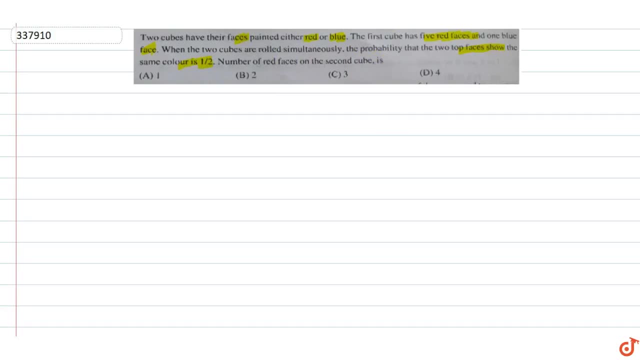 shown on the top face of the cube is 4.. On the first cube the number of faces on the cube is 1.. We get four, two família. Let us compare the faces of the first and second cube And let us see what is the face of the first cube. 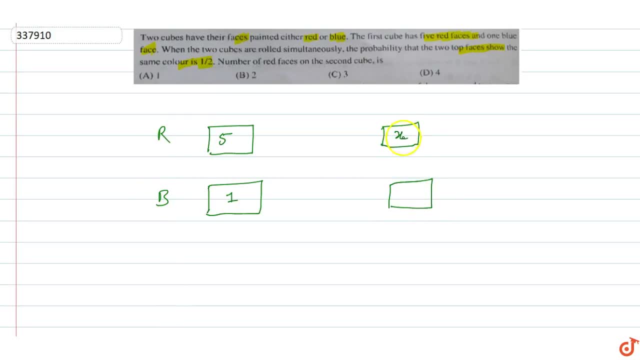 so, on this, what will be the blue x here? total will be red. so there are 6 faces on the cube, so remaining 6 will be on x. it will be blue. now what will be the probability of the red face on this? 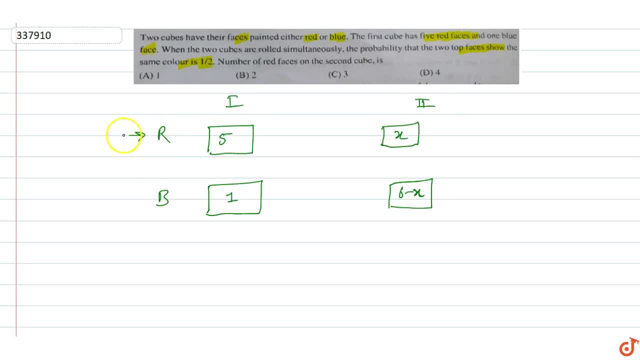 this is the first cube. this is the second cube. what will be the probability of the red face on the first cube? this is 5 by 6. we will choose one of the faces from 5, 5,, 7 and total. how many faces are there in the cube 6? 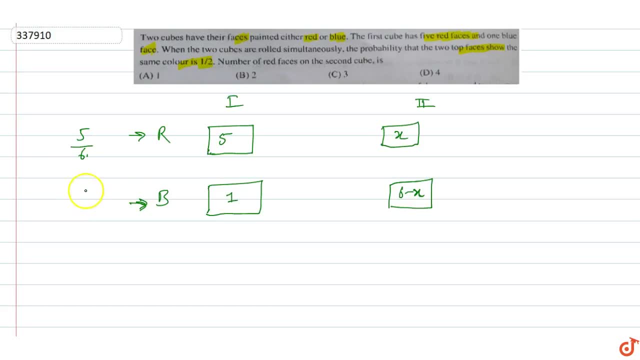 so 5 by 6. only one face is blue, so 1 by 6. and in the second cube, x faces are red. so what will be the probability of the red face on the cube? this is x by 6, x by 6. and what will be the probability of the blue face on the cube? 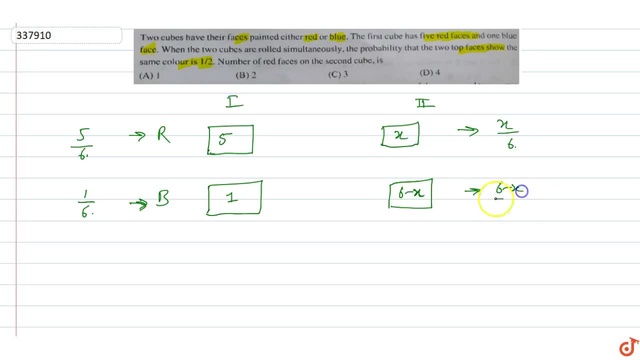 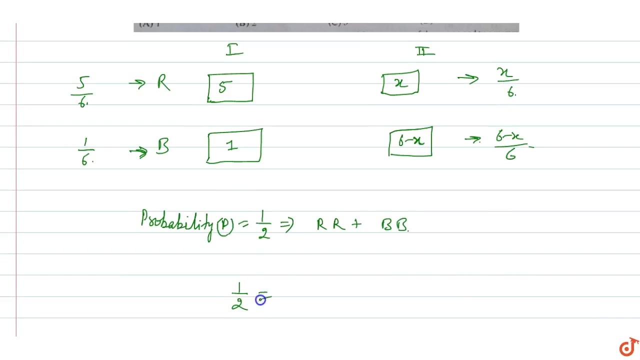 so 6 minus x are blue faces and total. how many faces are there? 6. so 6 minus x upon 6. now what is the probability of P? the probability of P is that two top faces when two cubes are rolled simultaneously. so what will be the probability of the red face on the first cube? 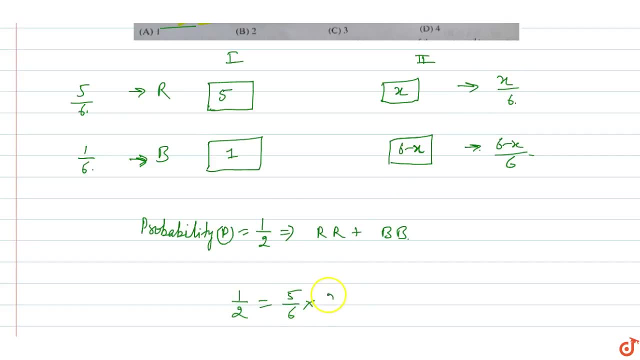 5 by 6 and what will be the probability of the red face on the second cube? x by 6 and what will be the probability of the blue face on the second cube? 7 by 6 and what is the probability of the blue face on the second cube?